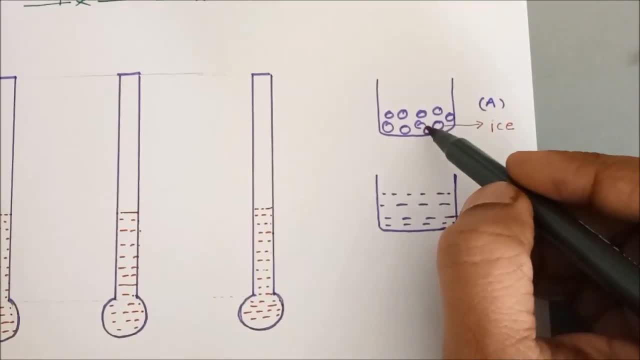 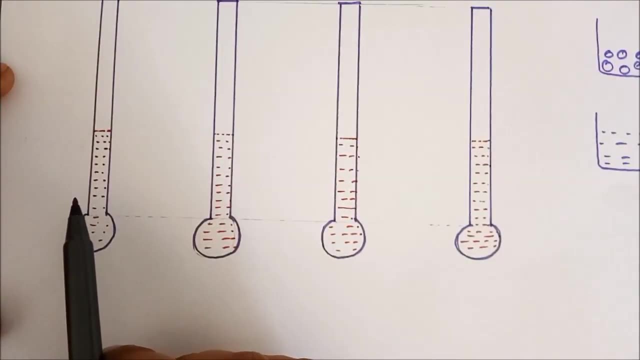 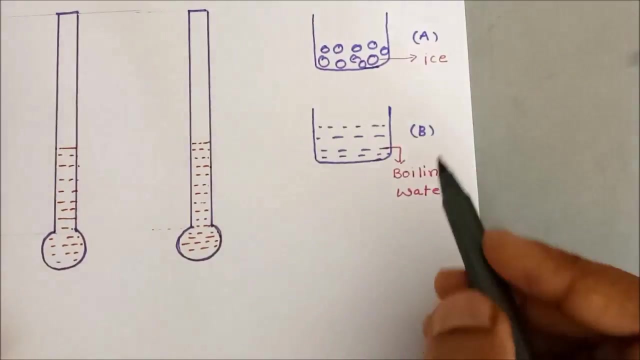 have another two containers, in which one having ice and the another one has boiling water. Let us assume that we all we keep all these four identical glass tubes which are having mercury in them. We dip it in boiling water. So what is going to happen? The mercury is going to absorb the heat energy. 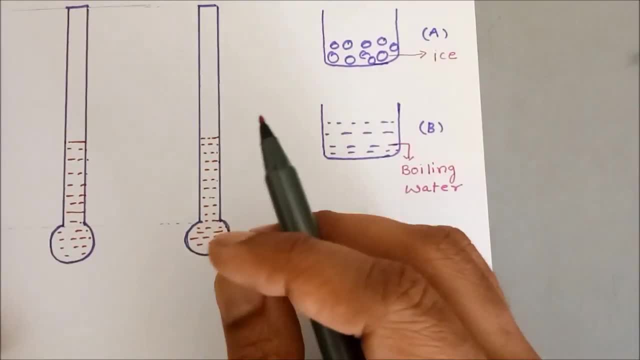 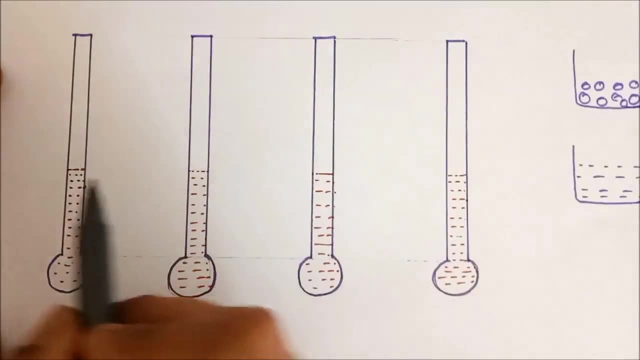 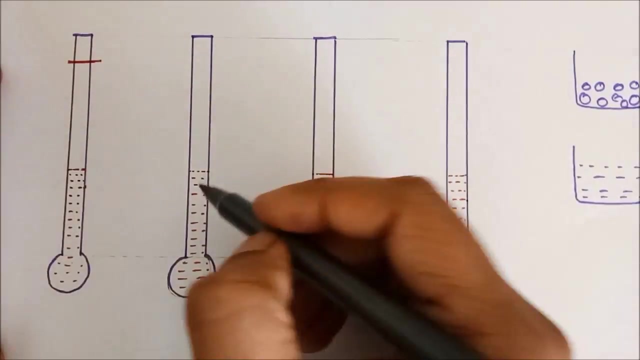 from the boiling water and since the mercury becomes hot, mercury will expand On expansion. you will see that this mercury climbs up and let us say the mercury reaches over here at this level. But since the all four containers are having same amount of mercury, all four containers are identical. So you will see that the increase in this amount of mercury, all four containers are identical. So you will see that the increase in this amount of mercury, all four containers are identical. So you will see that the increase in the 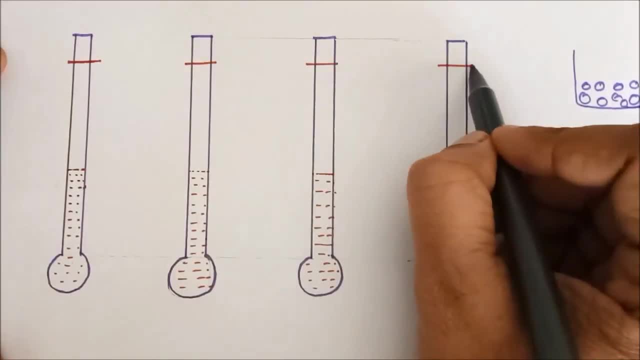 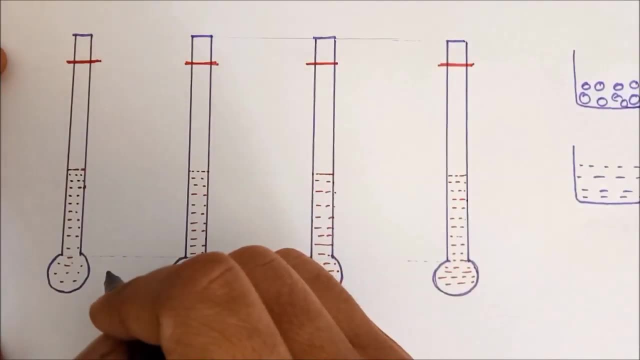 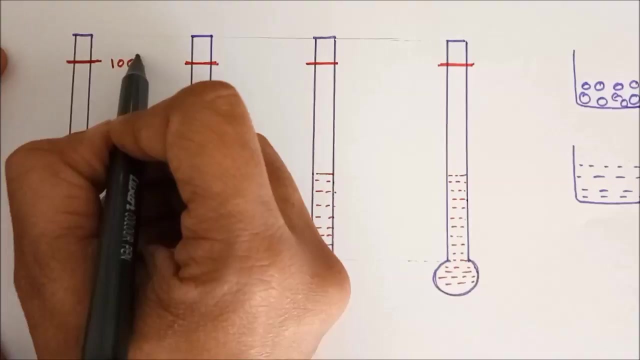 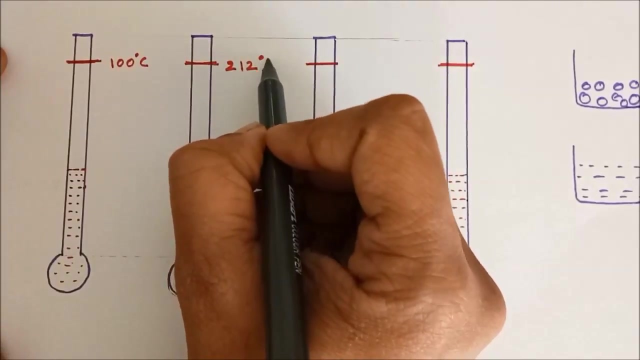 length will be same in all four. So these are the final heights at which the mercury is going to climb Now. celsius gave this marking as 100 degree celsius Fahrenheit. give this marking as 212 degree fahrenheit. Kelvin gave this marking as 212 degree fahrenheit and reservation. 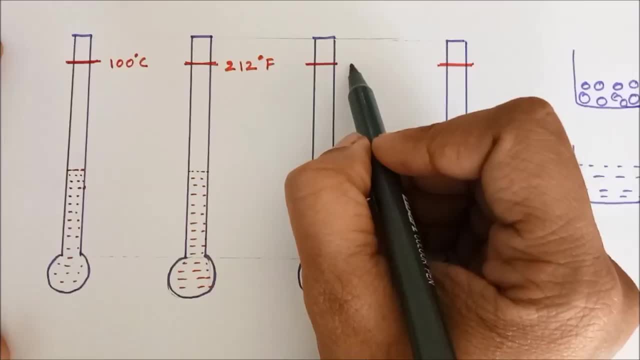 a 1 over 2 is what we get for celsius. Now celsius gave celsius as 1 over 2. where celsius gave celsius as 1 over 2 and the distance, which might be an compression, celsius name was changed. 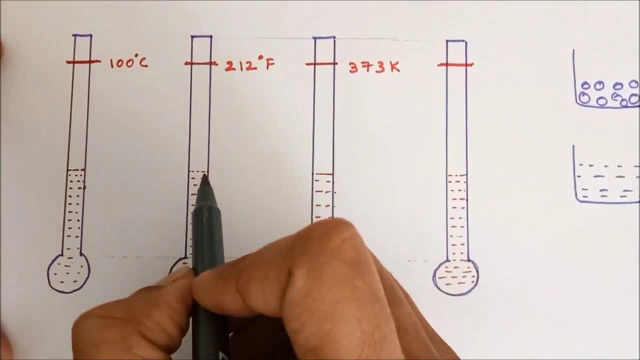 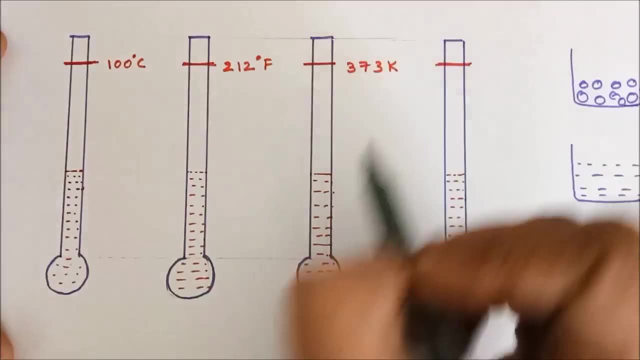 to cெ l, Now celsius gave the sameumin theme. Or how about watt per m and the temperature is? Make sure that we always say degree Celsius, degree Fahrenheit, we say degree Kelvin, but we never write down degree K over here. 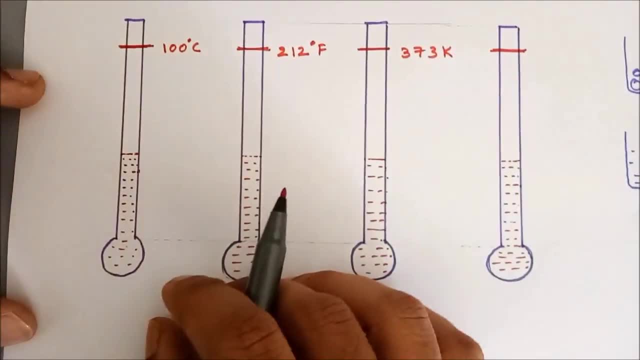 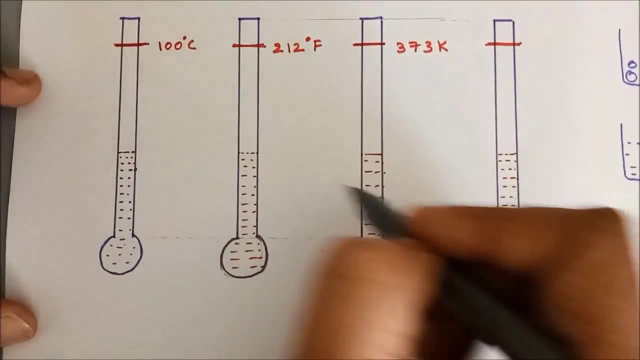 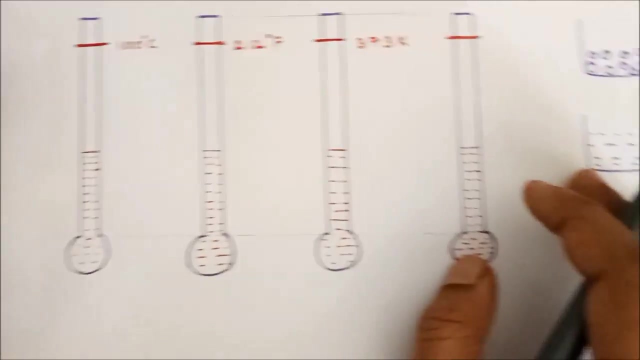 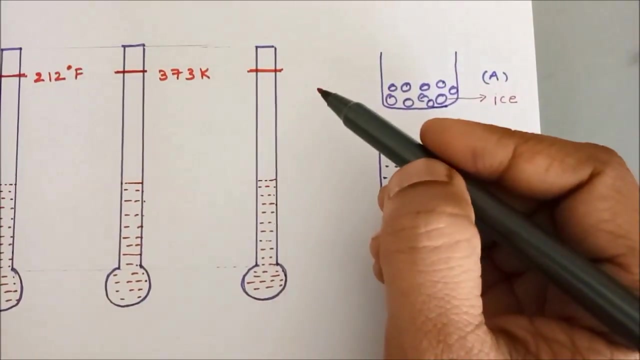 Let us keep this fourth as it is. Okay. now these are the final readings, or final lengths at which the mercury is going to climb. Now again, put this all: four identical glass tubes in glass. So what is going to happen? The ice is at lower temperature, the mercury is comparatively at higher temperature. 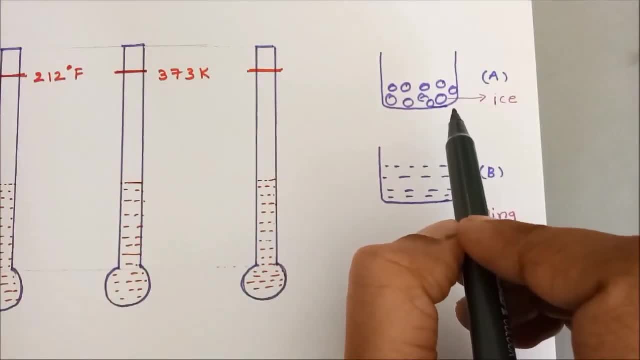 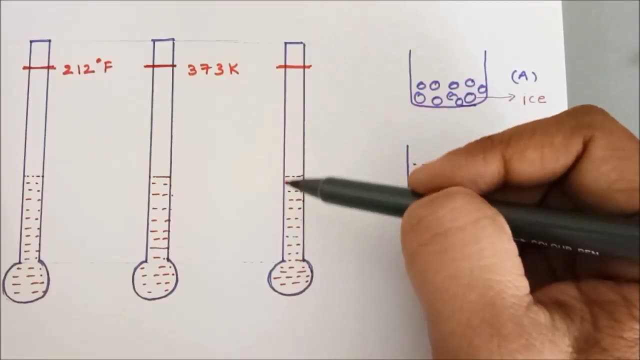 So the heat will transfer from higher temperature to lower temperature, So the mercury will start cooling and the mercury will contract. So what is going to happen? The level of mercury is going to decrease. Let us assume that the final level of mercury is this. 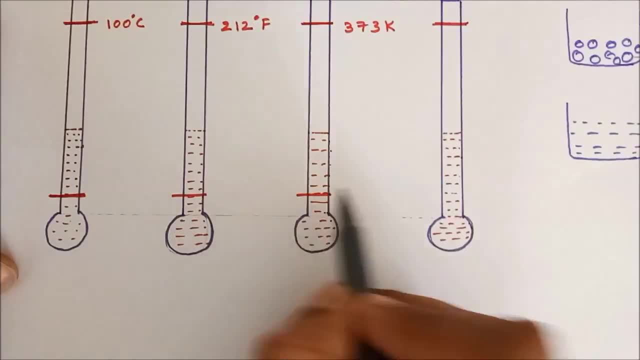 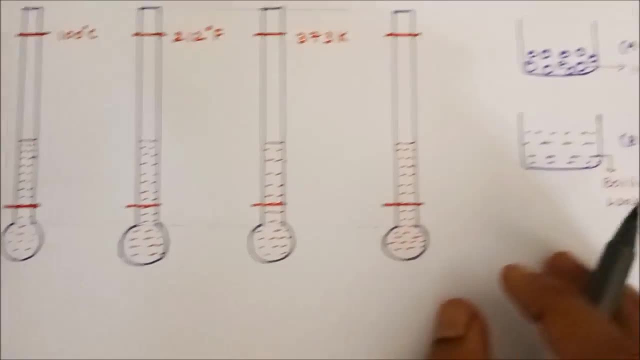 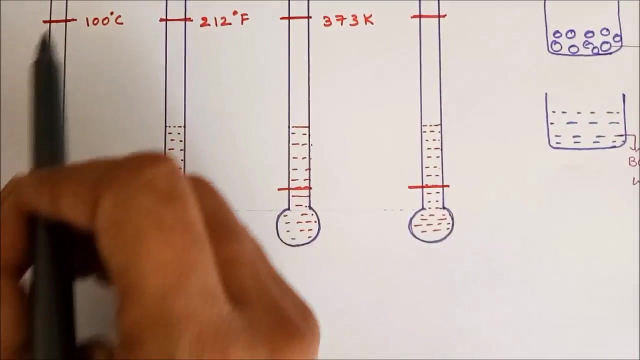 Why this has happened? Because the mercury was already expanded till this height because it was in boiling water. But if you put it in ice, the mercury is going to contract. and now, since all four are identical, whatever is going to happen over here, same is going to happen in the other three containers. 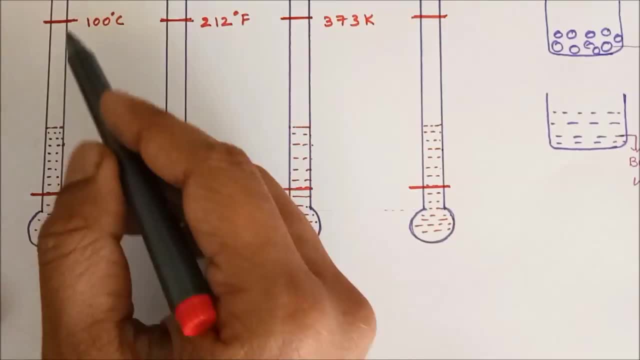 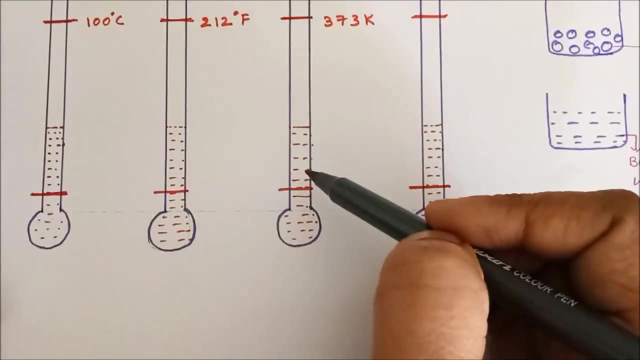 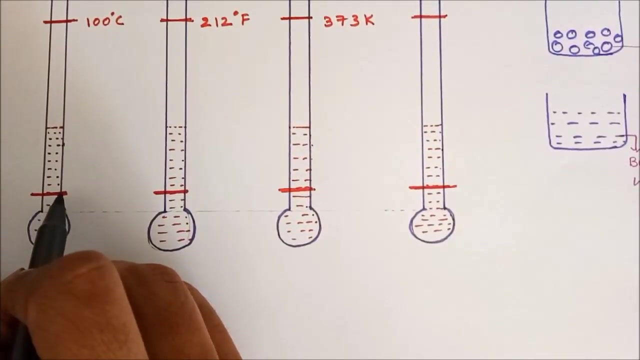 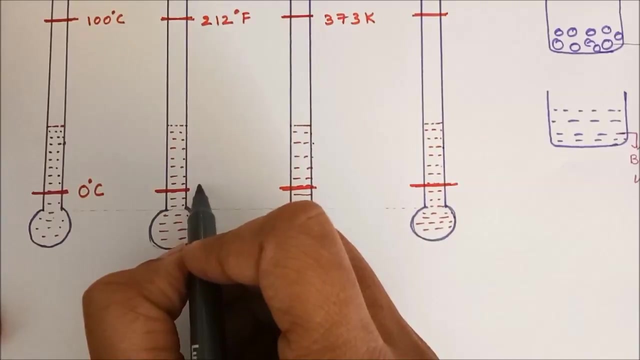 as well. So the mercury reading actually went down and came over here. So in all the other cases also, In the all other containers also, the mercury level fell down and these are the final levels of the mercury. This temperature reading was given: 0 degree Celsius by Celsius and this was said to be 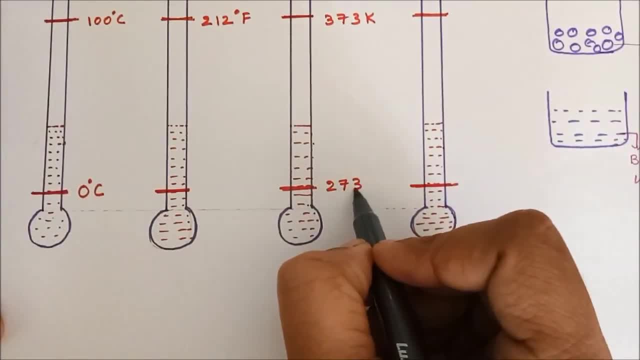 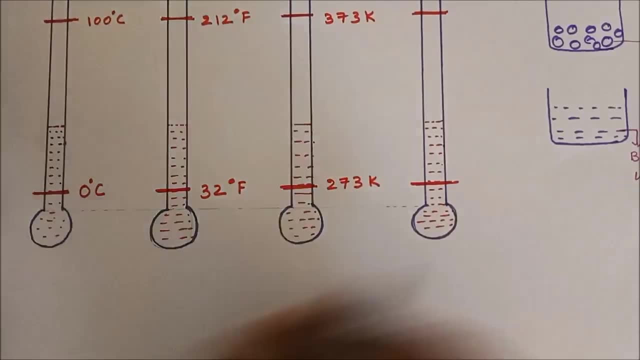 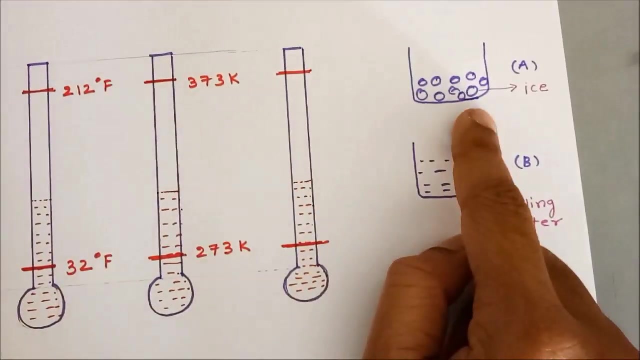 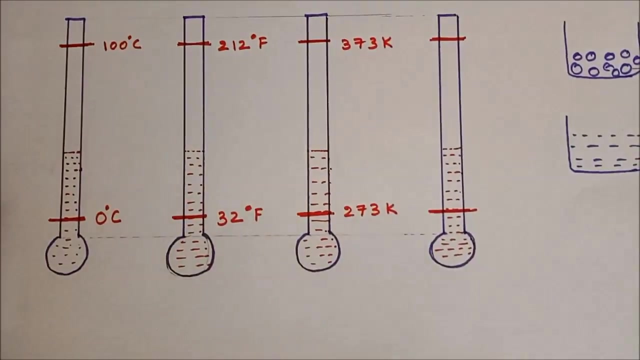 at 273 Kelvin by Kelvin, and this was said to be 32 degree Fahrenheit by Fahrenheit. So if you look carefully What has happened over here? By putting all these four vessels in ice and boiling water, we saw that the mercury went up till here, and the mercury went down till here. 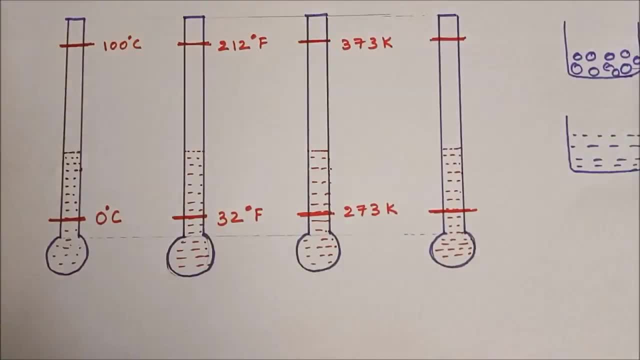 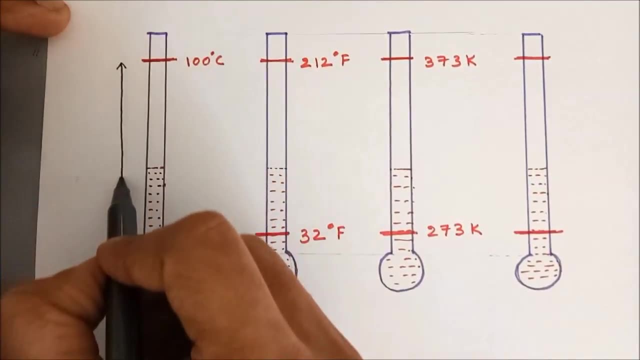 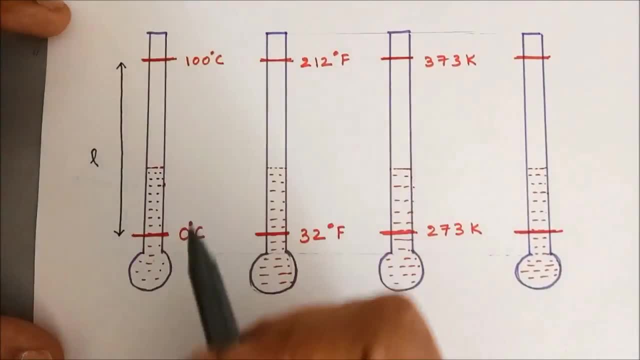 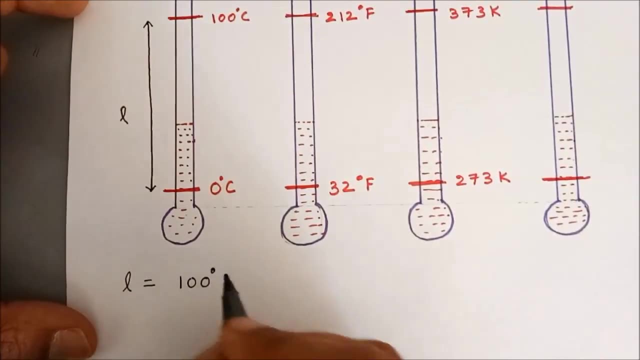 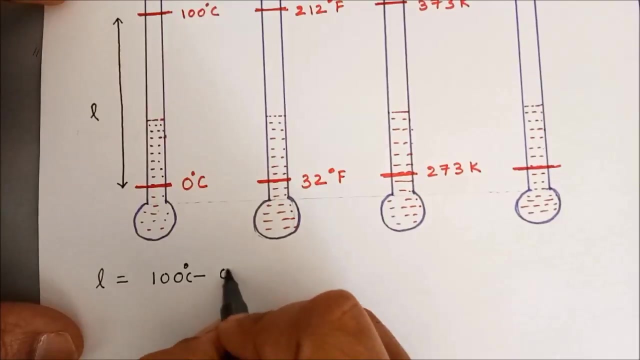 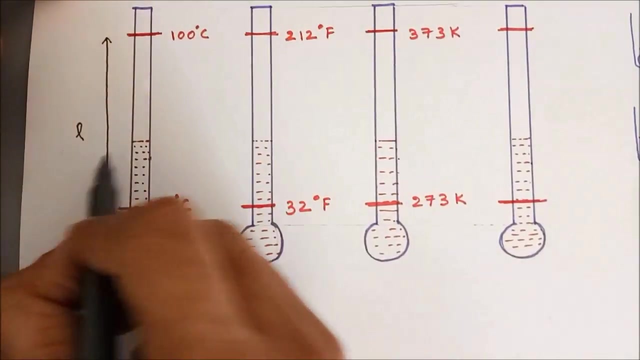 Now this length, L, is same for all of them. Now, in terms of temperature reading, I can define this length as difference in the upper point minus difference in the lower point. Here for the Fahrenheit scale, I can say that this length is again same over here, L. This 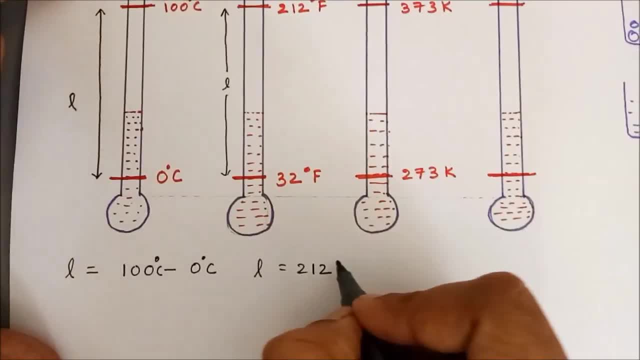 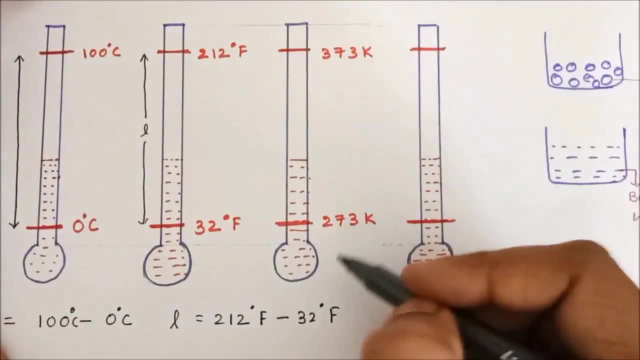 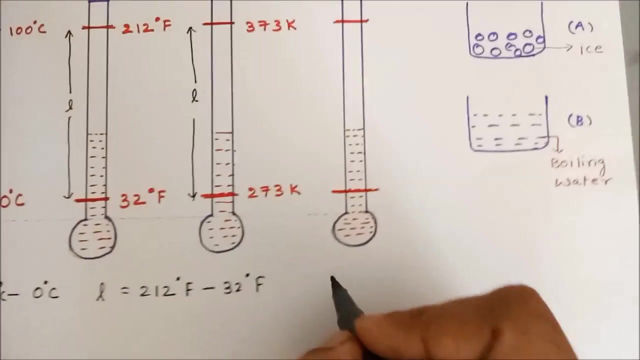 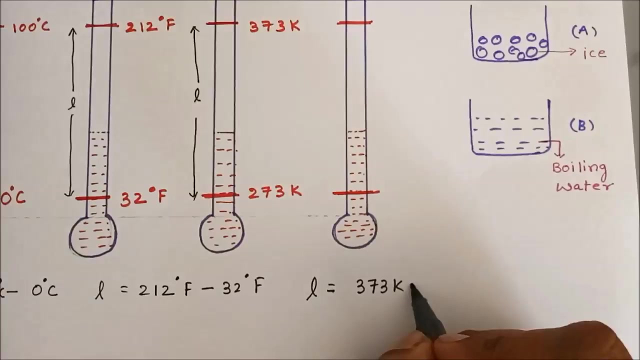 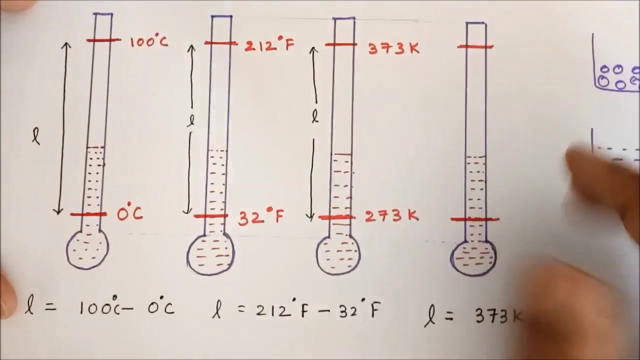 L is equal to 212 degree Fahrenheit minus 32 degree Fahrenheit. For Kelvin scale, this length again is same. this length L is equal to upper point 373 Kelvin minus 273 Kelvin. So let us once again, us once again- understand what we have done till now. We saw that when we dip all these 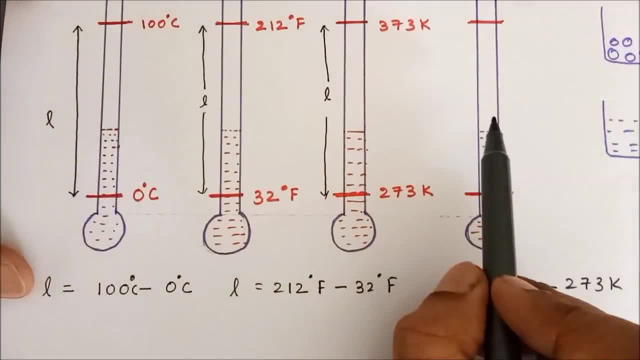 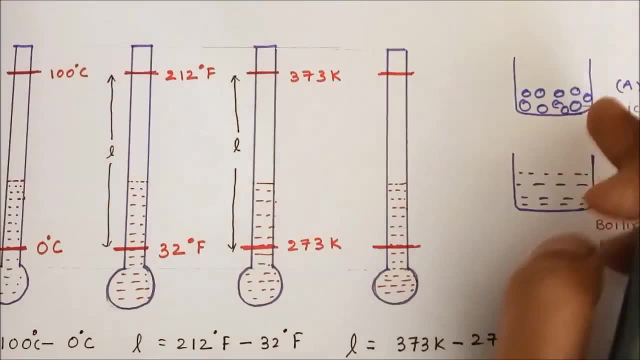 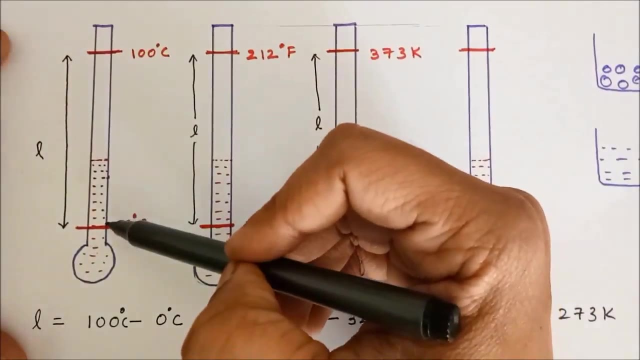 four equally filled, mercury identical containers. if we dip them into boiling water, the mercury level goes here, and if you put it in the ice, the mercury level goes down and comes over here. but this L length is the length by which the mercury went up or the mercury went down. 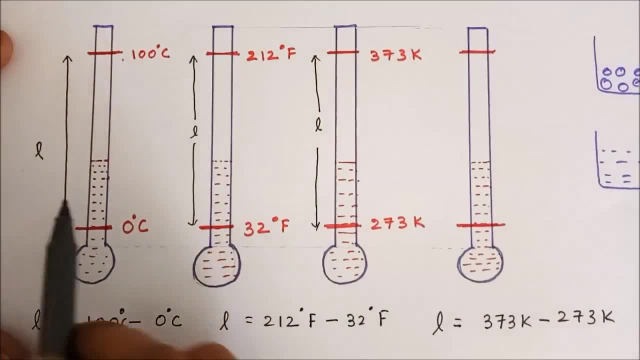 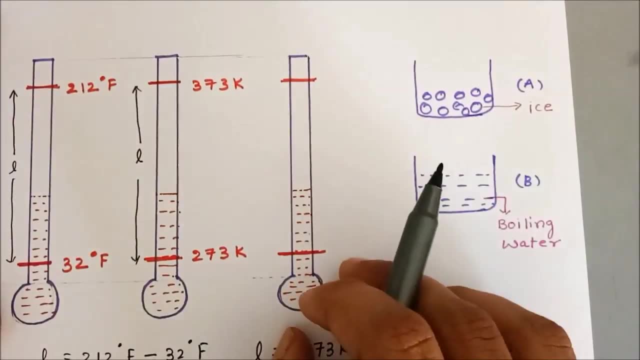 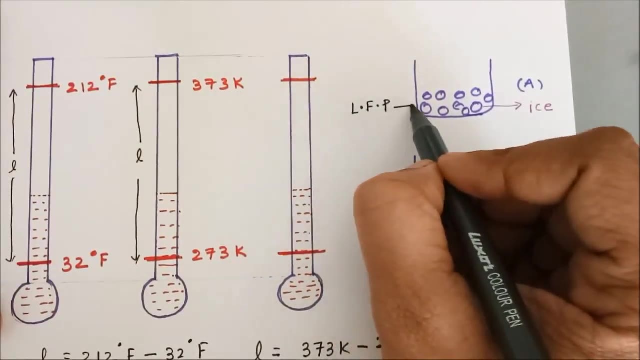 but this L is same in all the cases. It is because the containers are identical. same liquid is filled in all the four containers and these situations are also same for all of them. This is called the lower fixed point of the thermometer and this is called the. 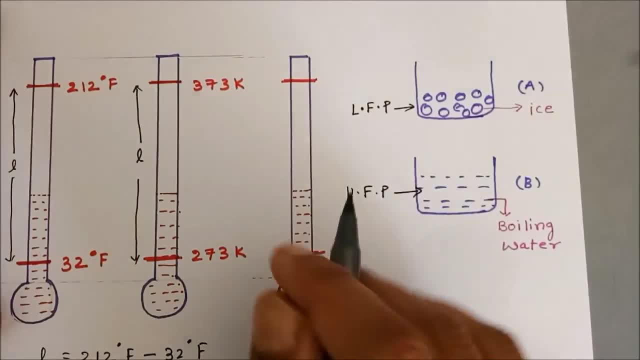 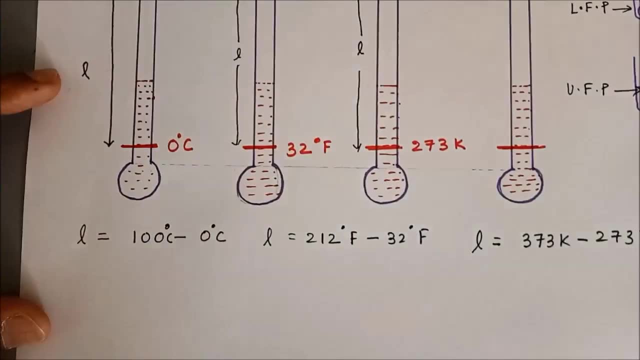 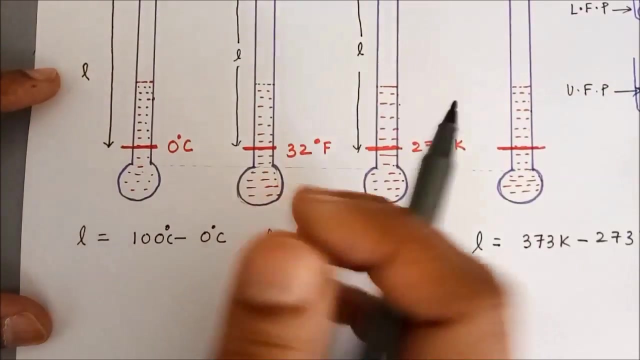 upper fixed point of the thermometer. We will come to know. we will study about this in somewhat more depth afterwards. Okay, Now let us assume that you have an imaginary vessel which contains some hot water at some temperature T. We don't know what the temperature T is. Now again, dip them all four in that. 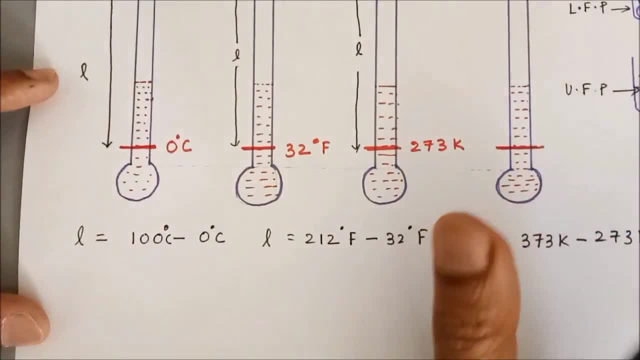 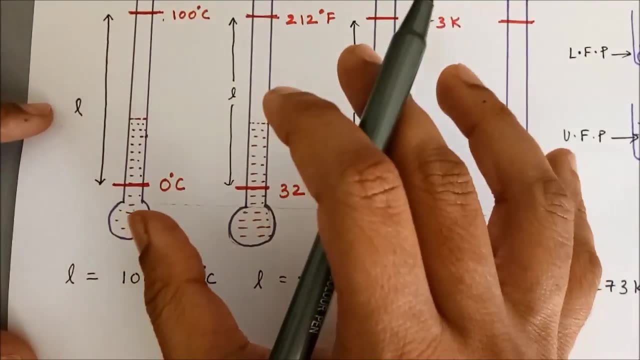 particular vessel which has got a water at some temperature T. That is quite hot, but not 100 degree. It is less than 100 degree and more than 0 degree. So let us assume that you have a vessel. that vessel contains water at 60 degree and we 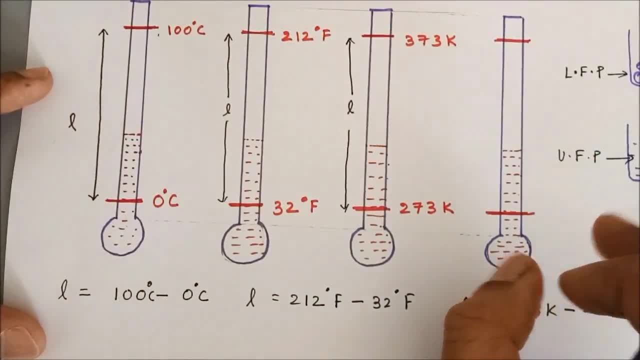 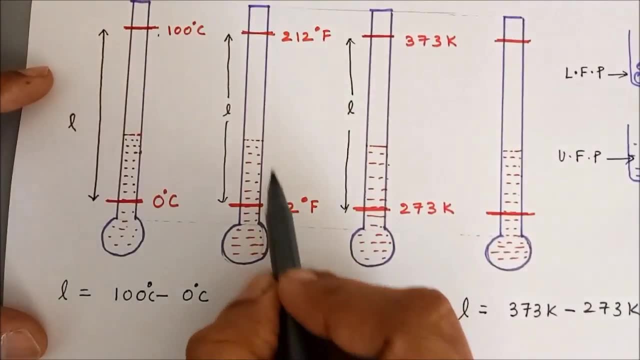 are dipping all these four containers in that vessel, having water at 60 degree. Then what is going to happen? The liquid level, the mercury level, is going to rise from here. It is going to rise from here. It is going to rise from here Again, it is going to rise from here. 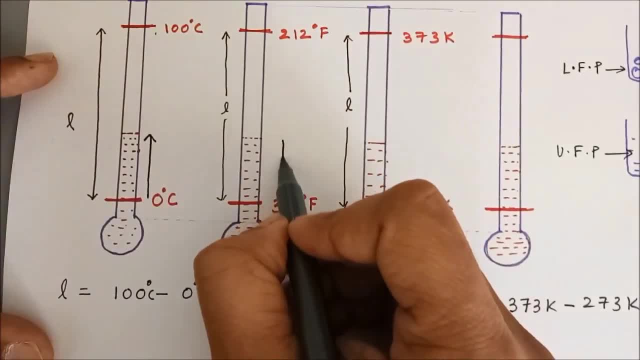 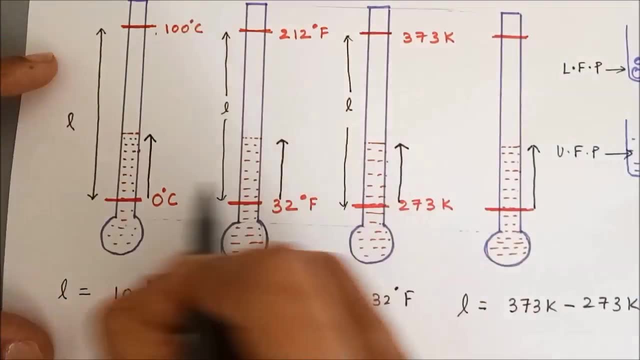 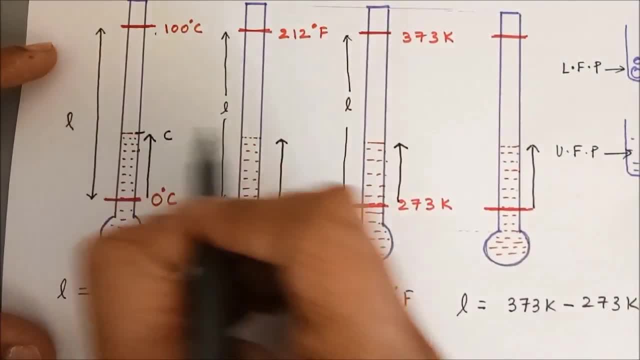 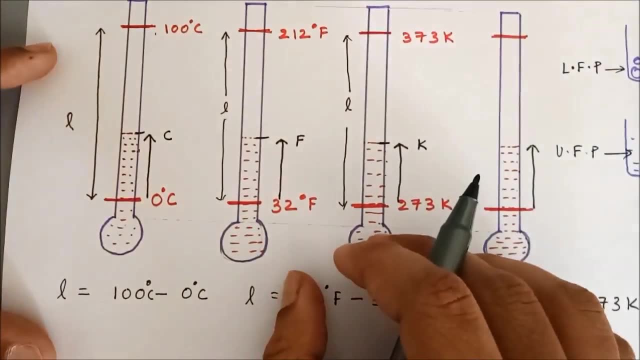 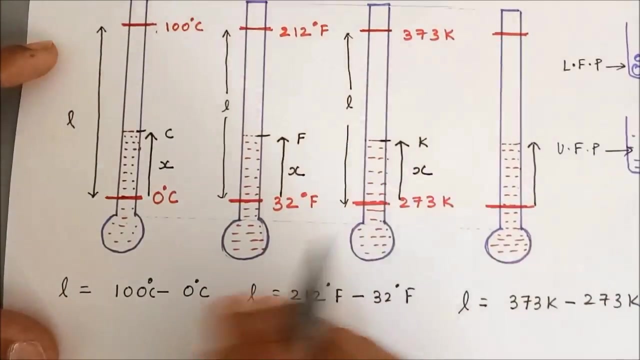 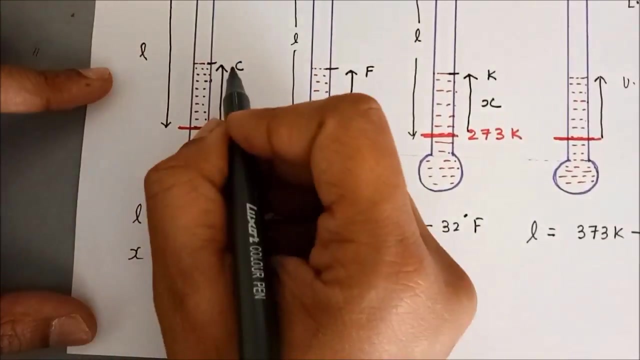 us see. Let us see the difference. Let us assume that mercury is rising. Let us assume this reading as C, This reading as F, This reading as K. Let us keep this as it is Now. this length by which the mercury went up is x x x. This x is actually difference of. 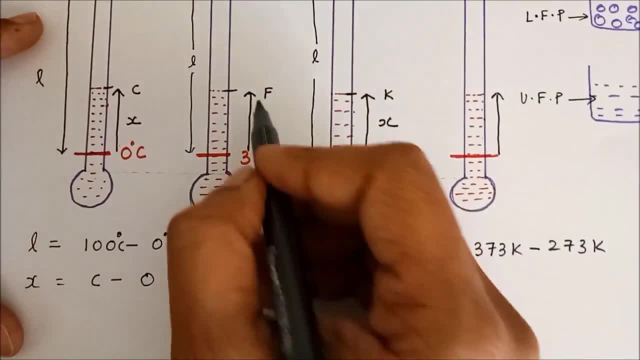 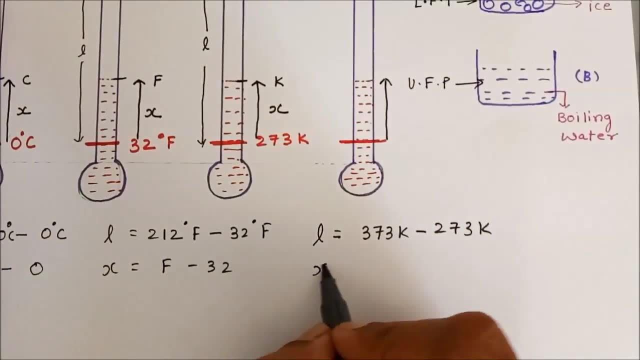 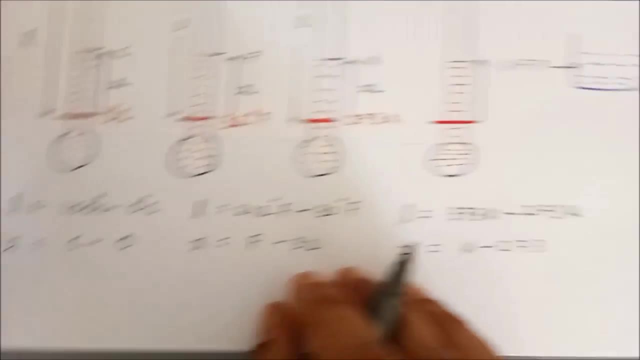 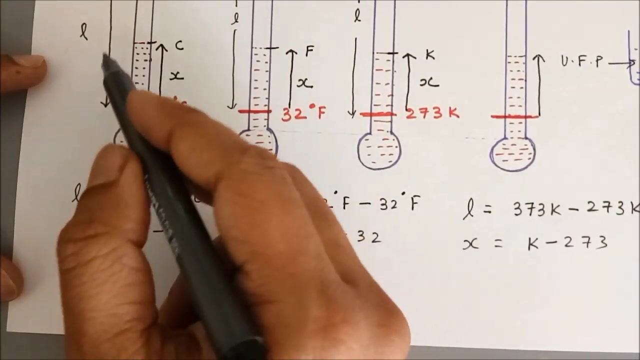 upper point minus lower point. Here the x is equal to. Here x is equal to k-273.. Let us find out the ratio. and we may also say that L is same in all 4, x is same in all 4.. 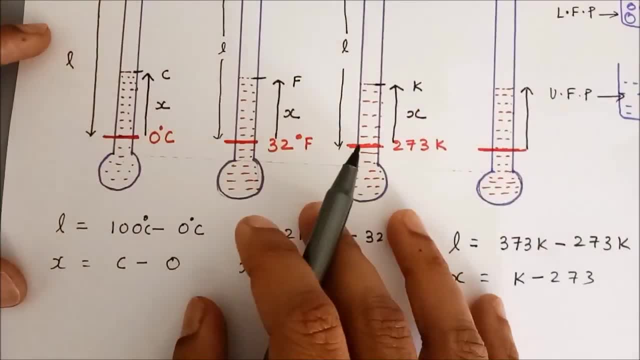 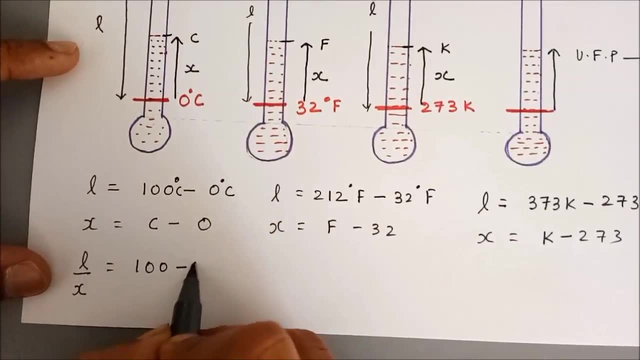 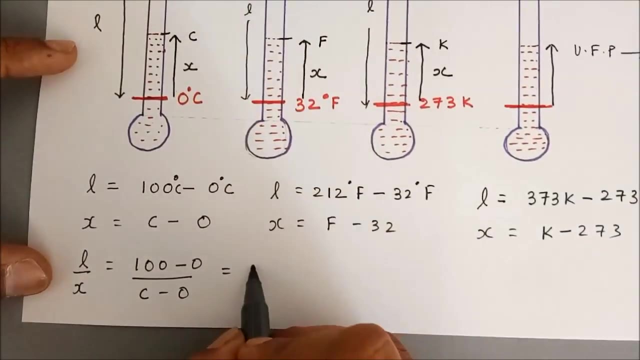 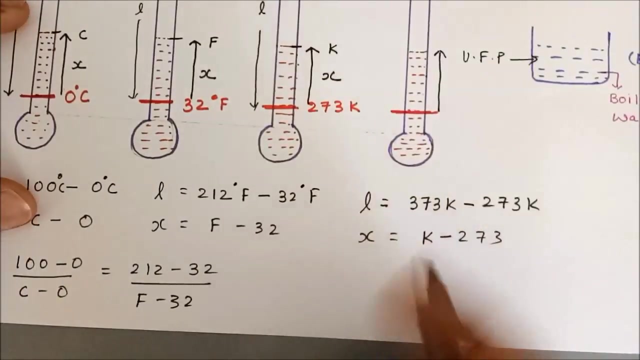 So if we find out L by x ratio in all the 4 cases, it will be same fine. So L by x ratio over here turns out to be 100-0 upon c-0.. That L by x ratio is same as this L by x ratio, that is, 212-32 upon f-32. 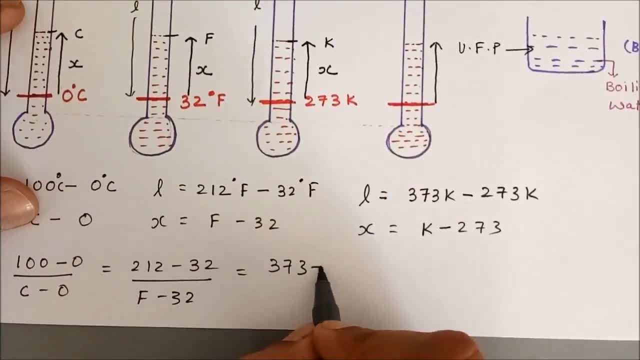 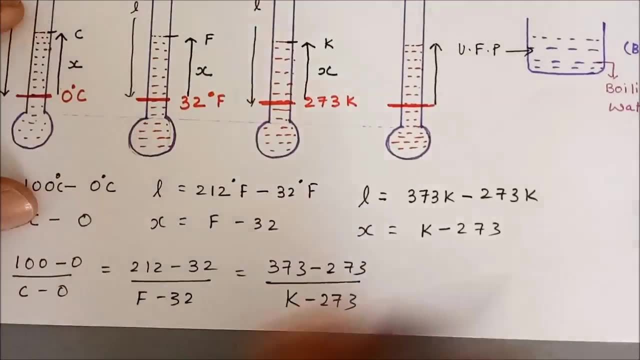 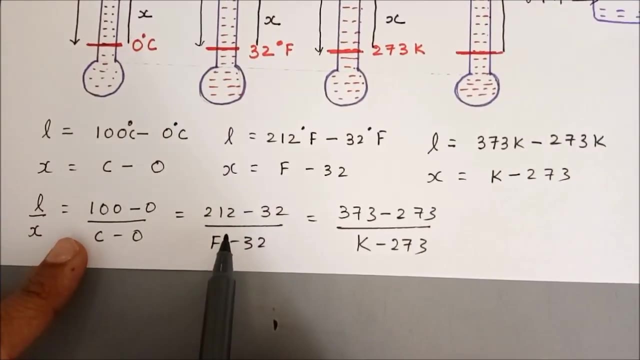 Here, L by x ratio is 373-273 upon k-273.. Okay, Now, if you compare any of these two, suppose, if you want to convert Fahrenheit into Celsius, then you can equate these two. If you want to convert Fahrenheit into Kelvin, we can equate these two. 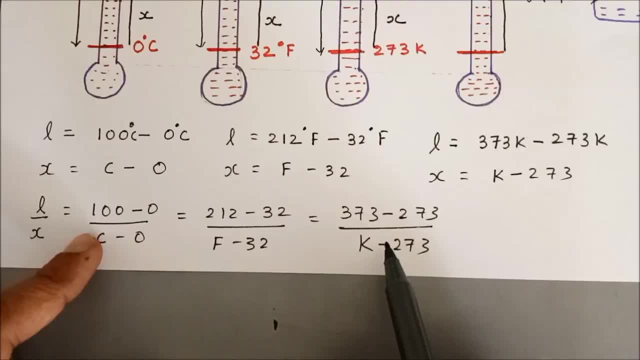 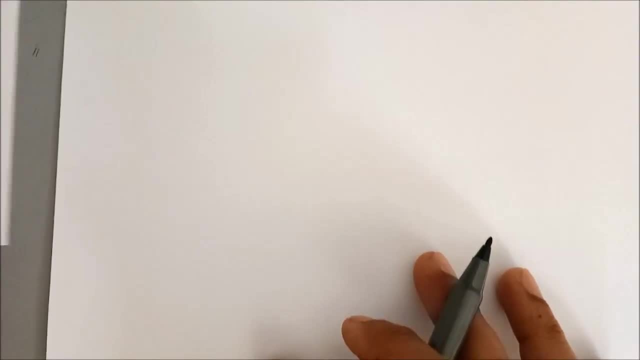 And if you want to convert Kelvin into Celsius, we can equate these two. So let us continue our discussion on the next sheet. So, finally, we had come up with this formula: L by x, that is equal to 100-0 upon k-273. 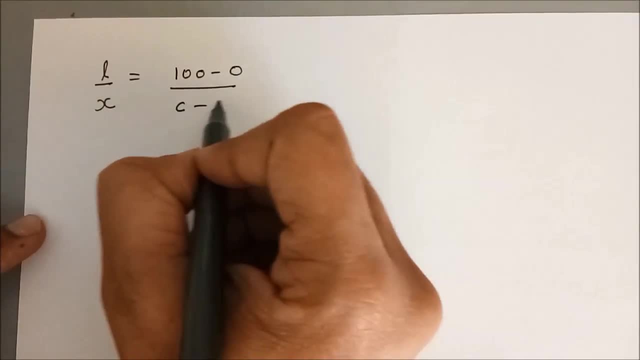 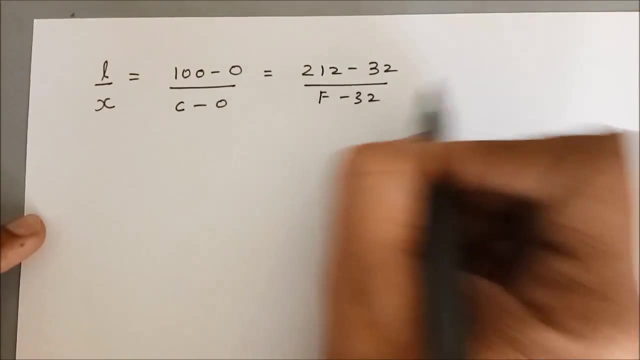 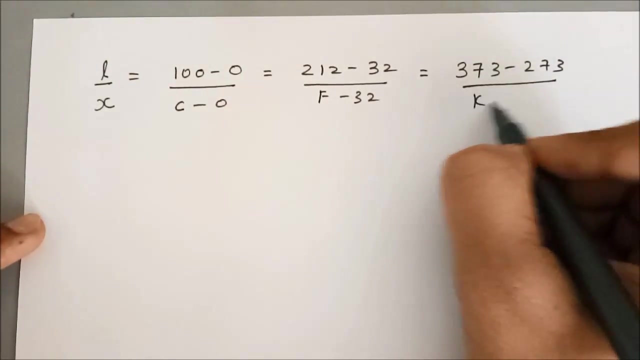 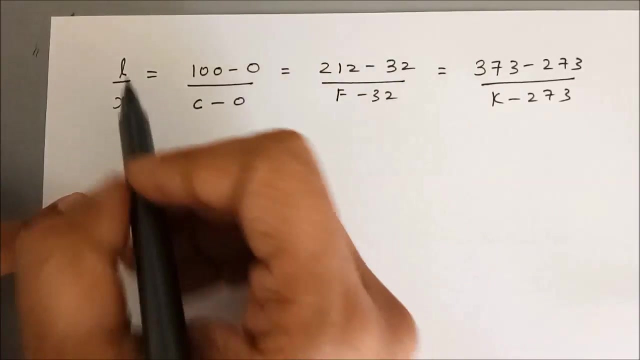 That is equal to 100-0 upon c-0.. That is equal to 212-32 upon f-32.. That is equal to 373-273 upon k-273.. Let us convert Celsius into Fahrenheit. So we are going to equate these two equations. 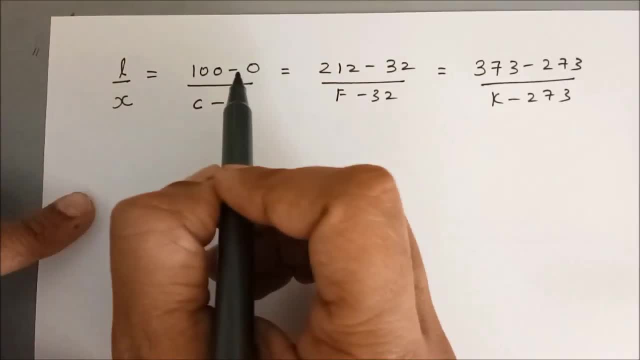 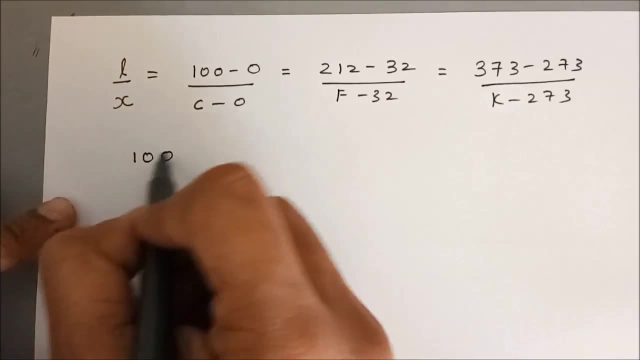 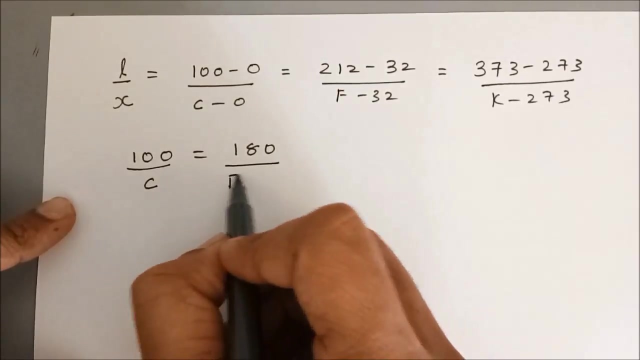 It is because L was same in all cases. x was also same in all 4 all the cases. so L by x ratio will be same for all the cases. So 100-0 is 100, c-0 is c, 212-32 is 180 upon f-32.. 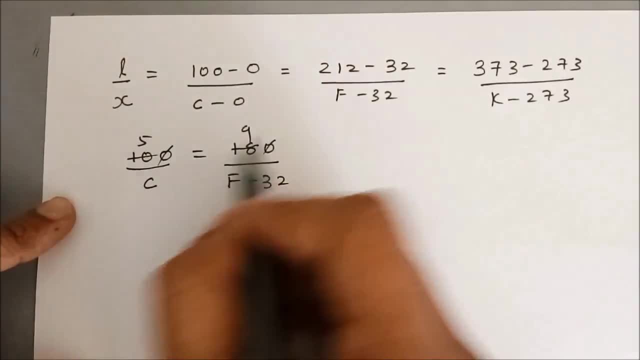 You can cut these two, two 5s, two 9s, and we can then cross, multiply and we can get our answer as 9 into c. that is equal to 5 f-32.. So c is equal to 5 by 9.. 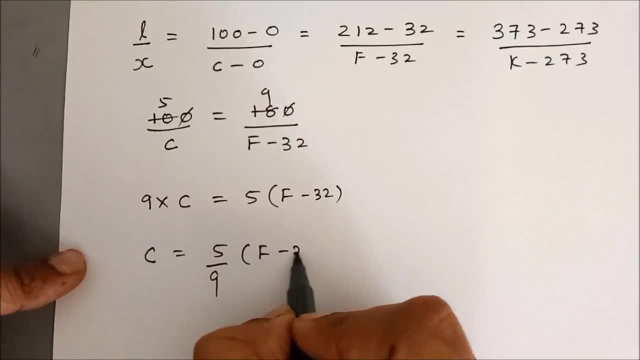 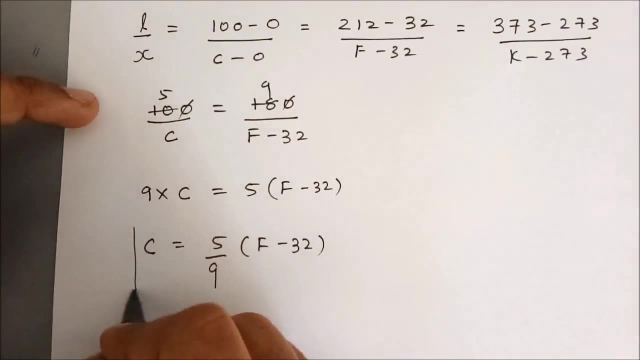 Okay, So c is equal to 5 by 9 f-32.. So here we come up with an very important formula. So I guess that we now need not to mug up for any kind of formulas in the exams. We can. if you even forget it, then you can also derive it in a small space. 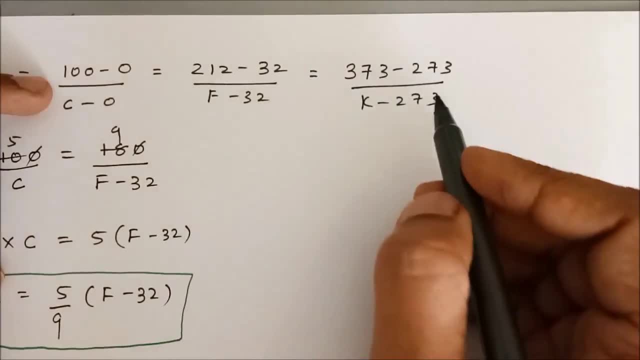 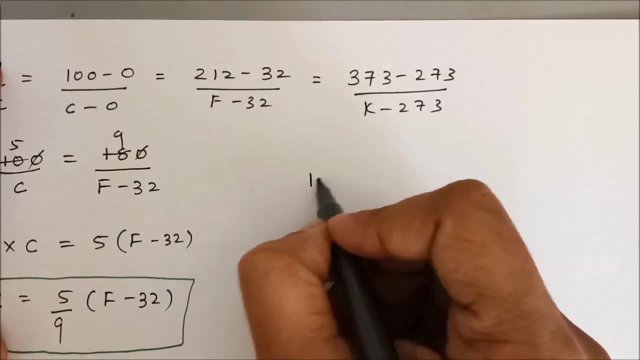 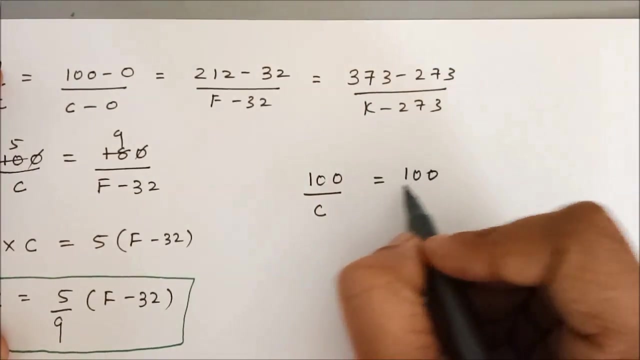 Let us also convert the Celsius into the Kelvin, So we are going to equate these two and here it is 100-0.. So that is 100 upon c, That is equal to 373-273, is 100 upon k-273. 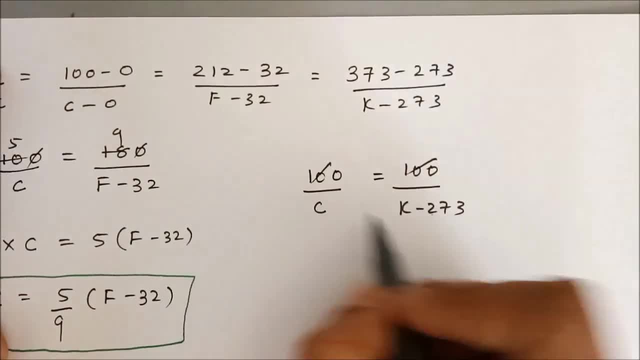 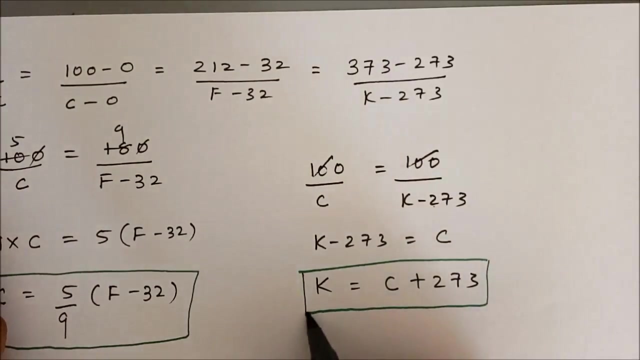 So these two gets cancelled cross. multiply here 1 into 1.. So k into 273, k-273 is equal to c into 1 is c, So Kelvin is equal to Celsius plus 273.. So here we also come up with another derivation. 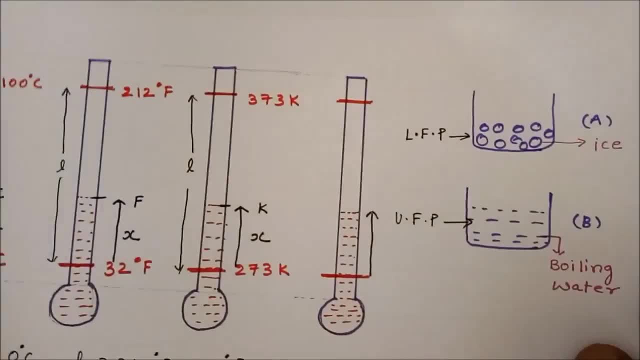 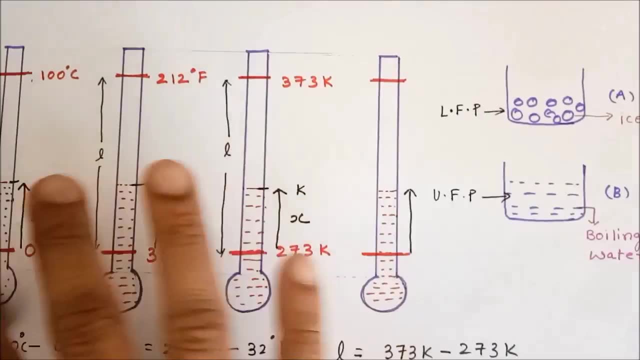 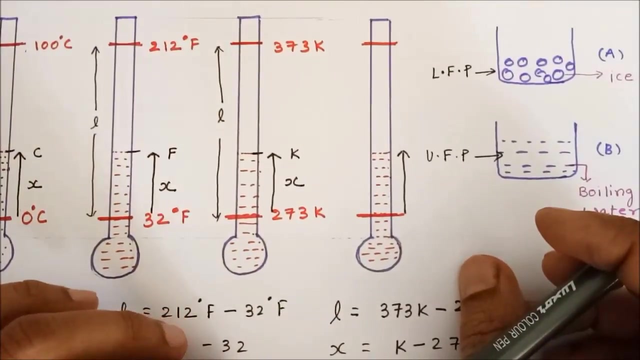 Now we may also wonder, Okay, That what is the purpose of this last one, last vessel in which there is mercury? and the same thing is happening over here. So I am going to make my own thermometer and I am going to give this thermometer as my 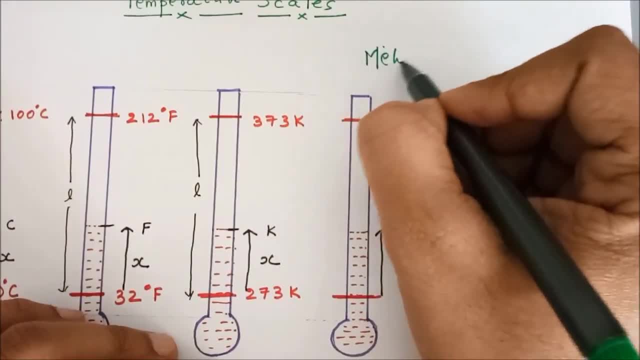 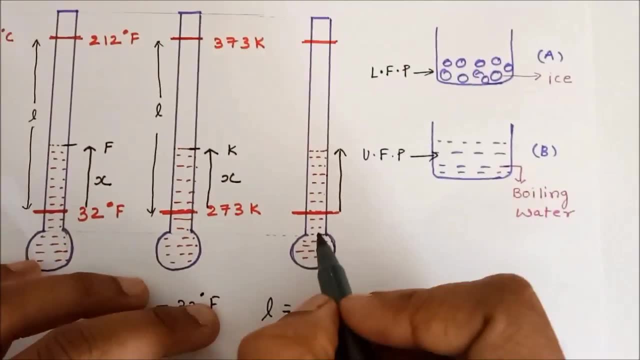 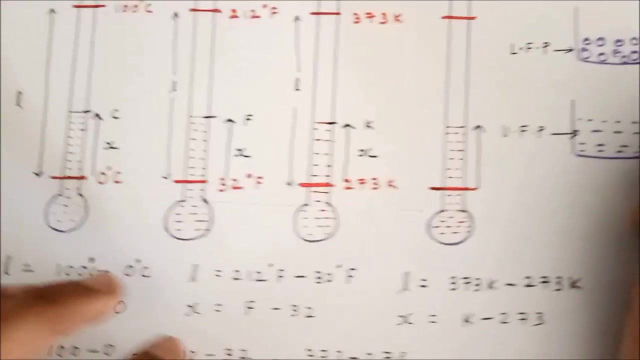 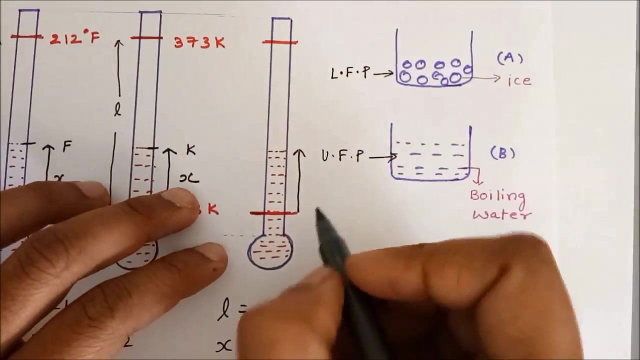 name, as this is my surname. Okay, Now I am selecting this point. Okay, So this is the melting point of ice, that is, the 0 degree as per Celsius, 32 degree as per Fahrenheit and 273 as per Kelvin. I am going to select any random number. 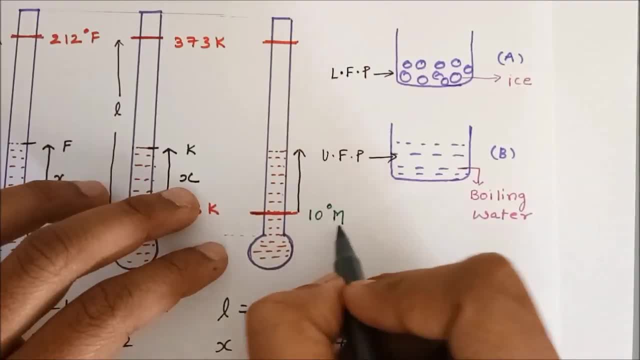 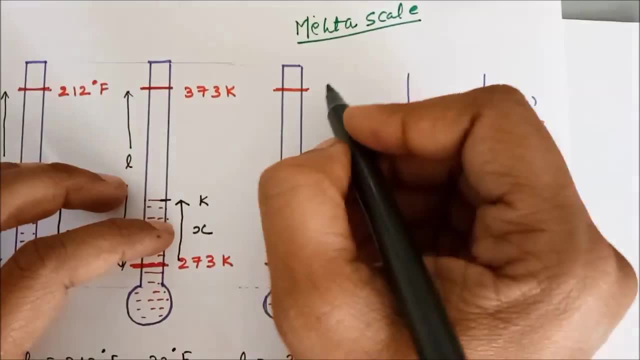 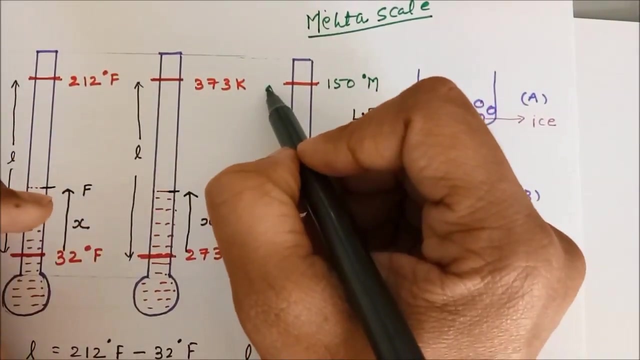 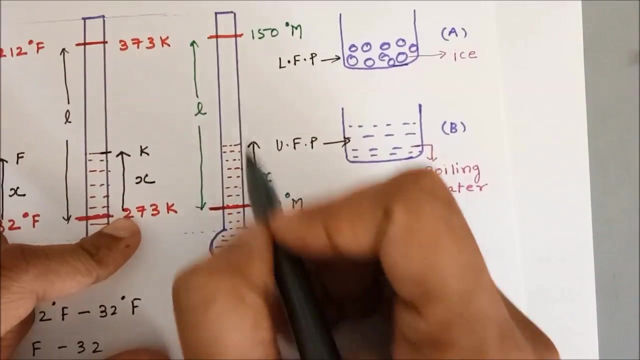 Let me call this as 10 degree m on my scale, and I can also select this boiling point of water as say, for example, 150 degree m. Okay, Okay, Okay. So this length l is again same as the other one, and this length x is also going to be.